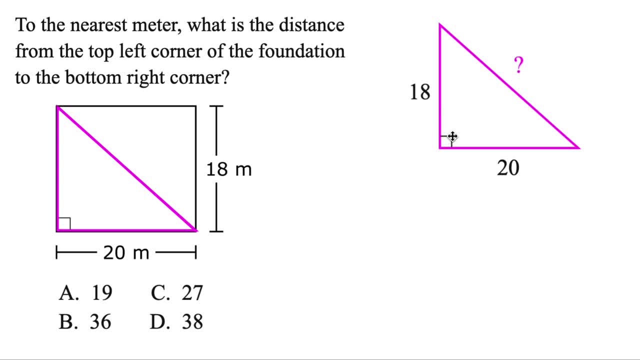 18 to the other side there. Now, if you have a 90 degree angle and if you know two sides of a triangle, you're trying to find the third. you could always use Pythagorean theorem If you're like, oh no, this looks a disaster, it's not that bad actually, You just have 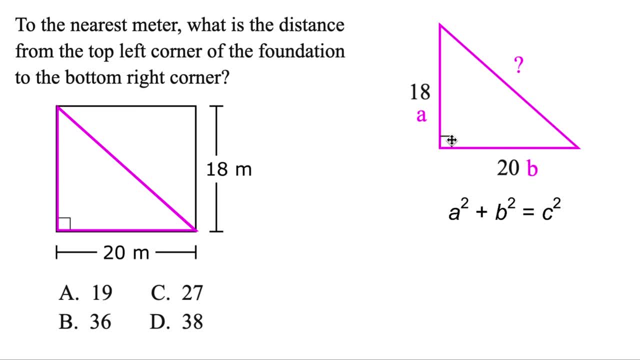 to label A and B. those are the sides that make up the 90 degree, and then this thing kind of looks like a, C, so opposite of that is where C goes there, And then from here, if you know A and B, it just turns it into an addition problem. So this is what we're. 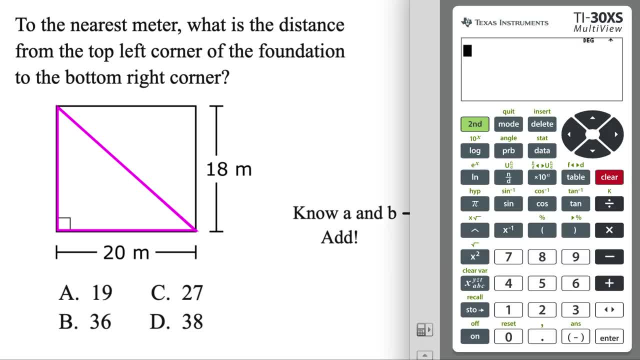 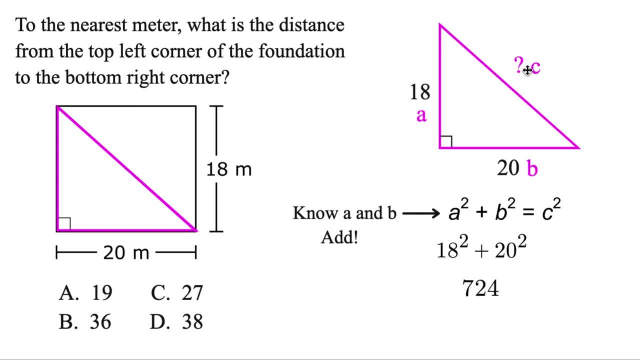 going to type into the calculator. to start here, Let's do it. Okay, we got our 18, squared and then plus 20.. We'll use that X squared button. Okay, that gives us 724.. Let's copy that. But obviously that side here C can't be 724.. That's way too big. So the 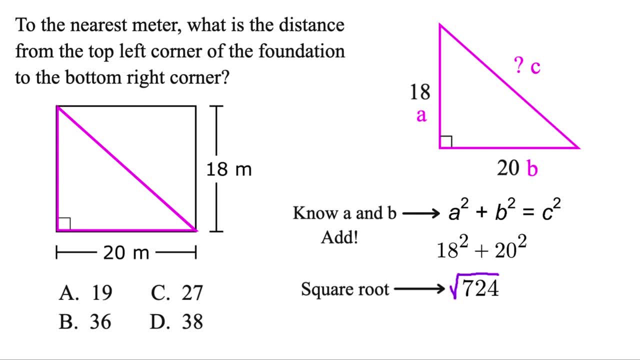 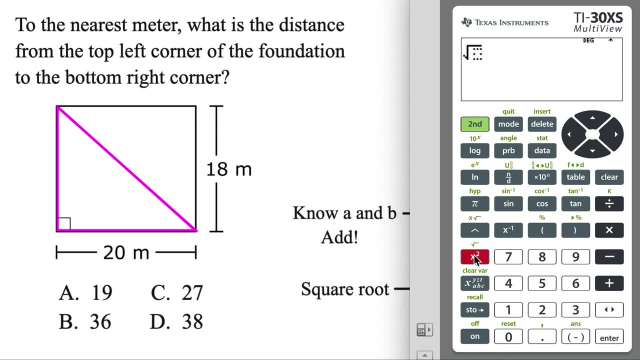 last step is: you'll always square root. to get the final answer here And to do the square root, you could always- let's clear, you'll do the second, then the X squared button, then type in what you want to square root. 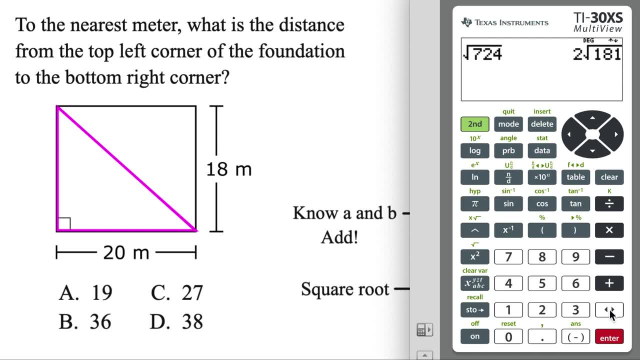 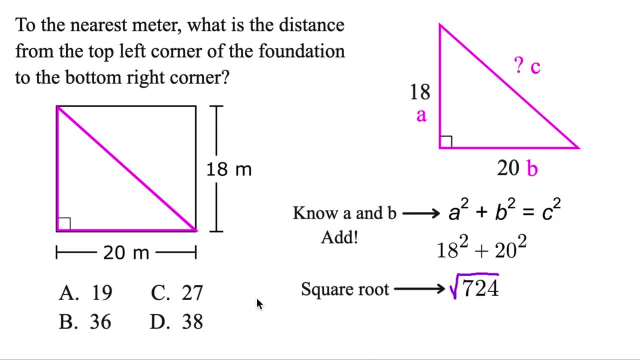 And boom. Now this looks a bit of a mess, but just hit the button above: enter. Same thing as 26.9.. So, rounding it up, our answer is C there. Therefore, that distance C is 27, and that distance there also 27.. Okay, let's look at another one Now. this is the. 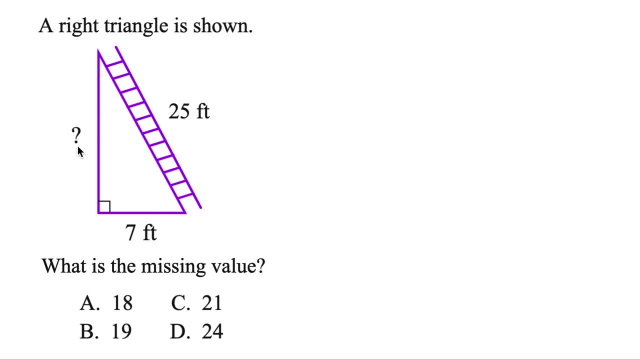 same idea, because we have two sides of a triangle. we're trying to find the third, so we're going to use Pythagorean theorem. Now let's label our A, B and C, But in this case, if you know, C. 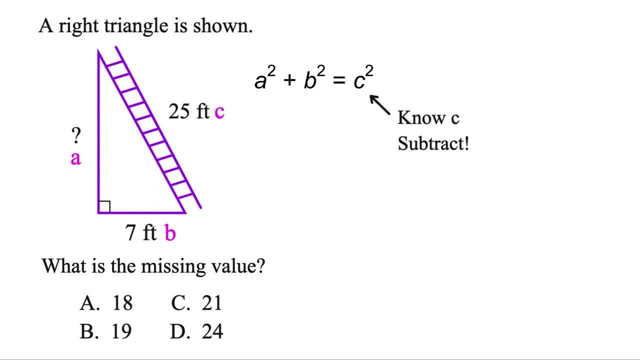 it's going to turn it into a subtraction problem. Why is that? Well, because this is the longest side, the hypotenuse C, but we're trying to find a smaller side, so we have to subtract to get there. Okay, so we'll start with 25 squared minus the other side squared. Now you could type that: 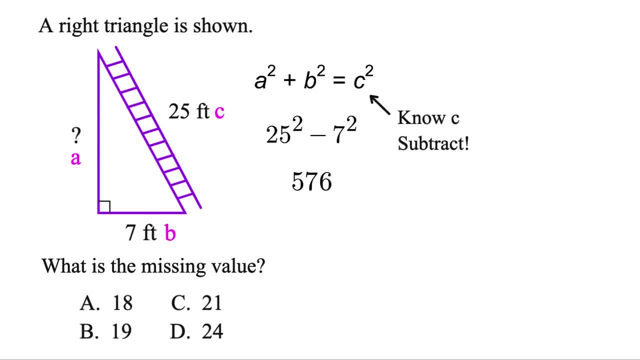 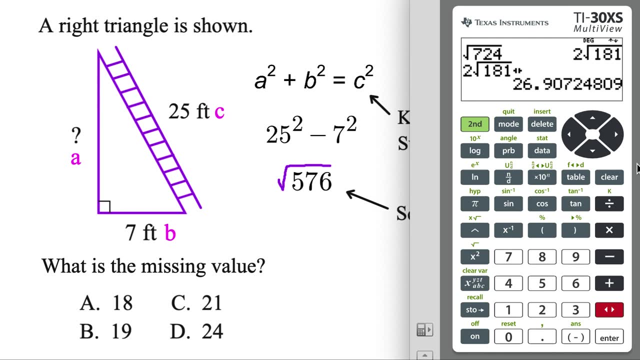 into the calculator. That'll give us 576, but way too big. so once again, square root, and that'll give us the final answer here. So let's see that. Okay, second X squared, then our 576,, boom, 24.. So that's our final. 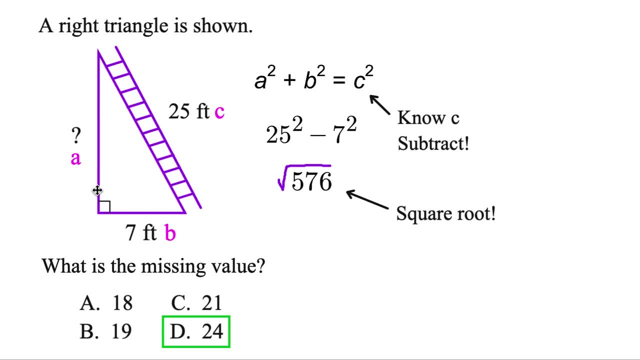 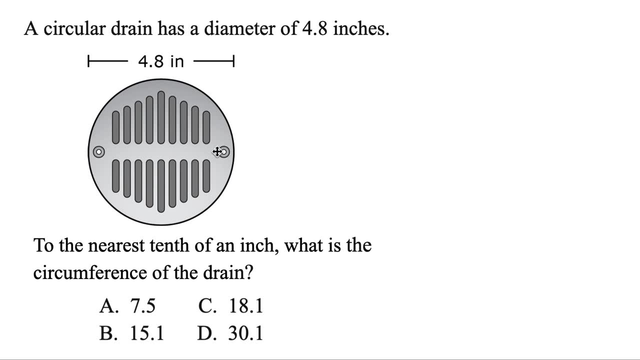 side and that's how high up along this building the ladder went: 24 feet there For this one. we're trying to find the circumference for the circle. Okay, so let's say we're going to do this all the way around the outside and they've given us 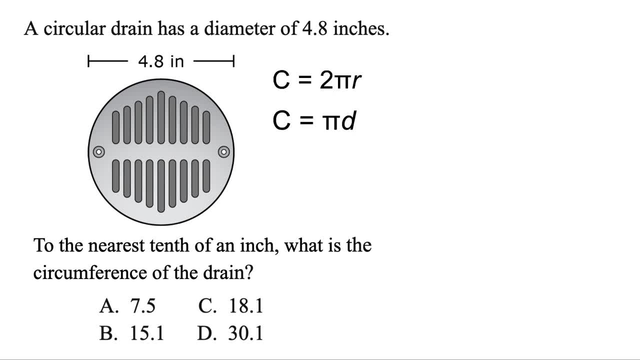 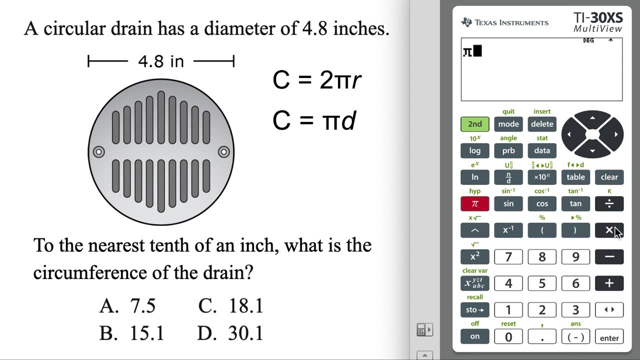 the diameter. Now this is where you're going to look up in the formula sheet and there's two equations for circumference. But because they've given us the diameter, we're going to trade that D, substitute it for 4.8.. So let's see what that gets us. Okay, we got pi times 4.8, our diameter. 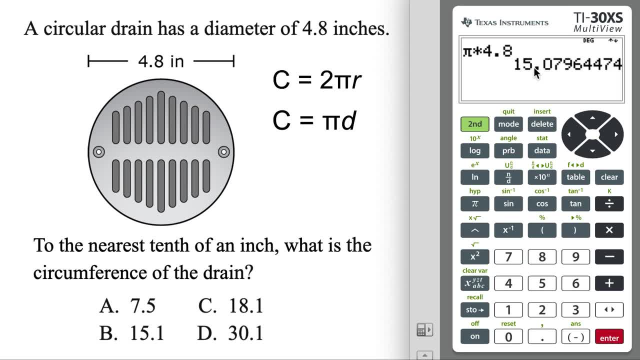 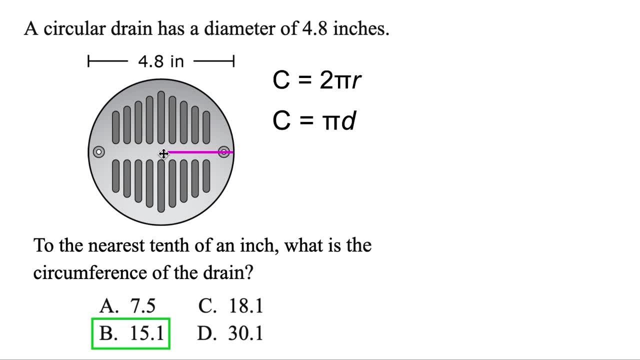 and that's it. Now you could just round it to 15.1.. So same thing as B there. Now, if they gave you the distance in pink from the center to the outside, the radius, then you would just plug in that distance in for R right there, and that'll give you the. 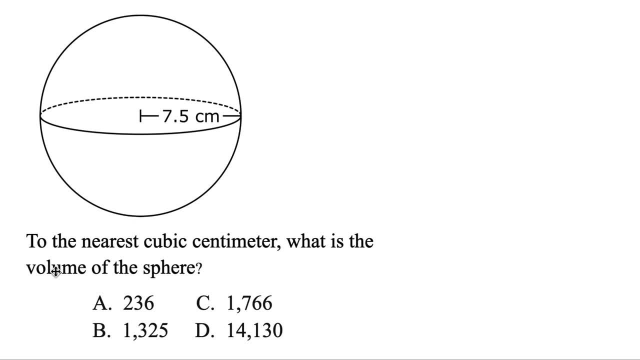 circumference This one, we're finding the volume for a sphere. So once again, we're going to use the formula sheet. We look that up and there it is. We're just going to change R, the radius, to 7.5.. So let's see what that gets us here. 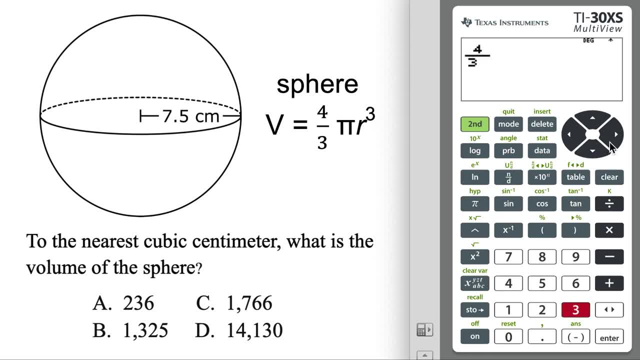 Okay, it's got a fraction. We got a 4 thirds. Then we have a pi, Then we got times, our radius 7.5.. And this one's to the power 3.. You'll use that up arrow 3.. Okay, that whole thing, 1767.. 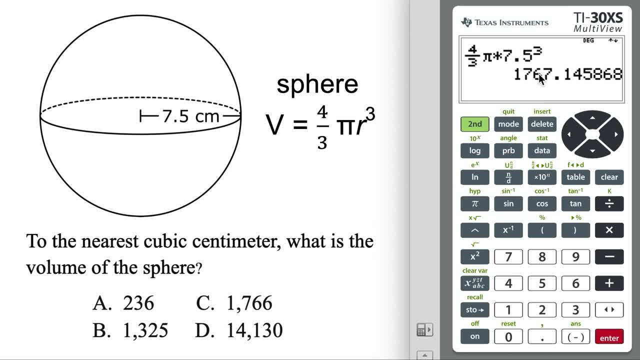 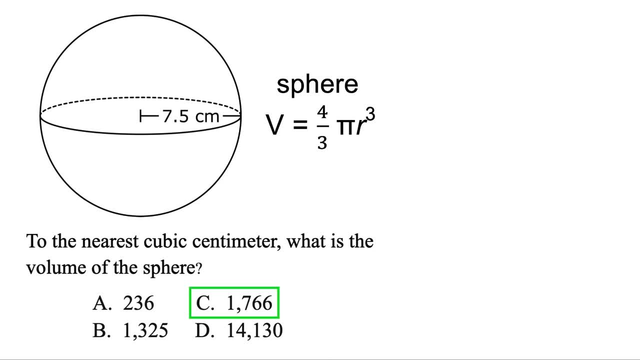 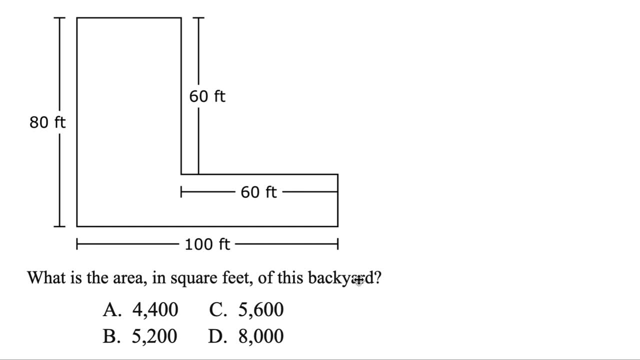 Closest answer is C. You might get a slightly different answer because they may use 3.14 instead of the pi button, But either way, it's going to give you the right answer there. And one last one: What is the area for this backyard? 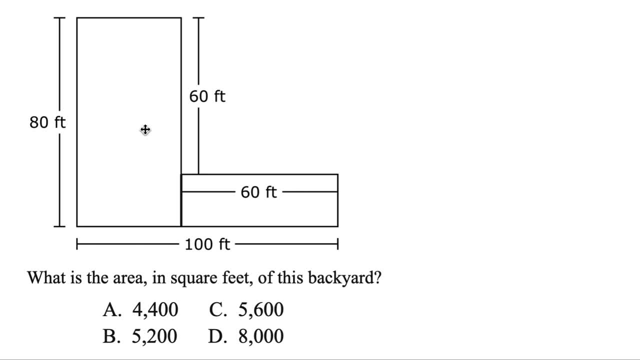 Now, right away, we're going to draw a line right there and turn it into two rectangles And we want to find the area for each of these and then add those together. But before we get there, we need to find this side length here. So let's label everything that.